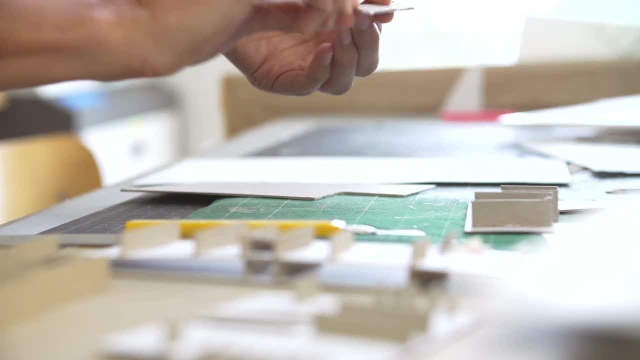 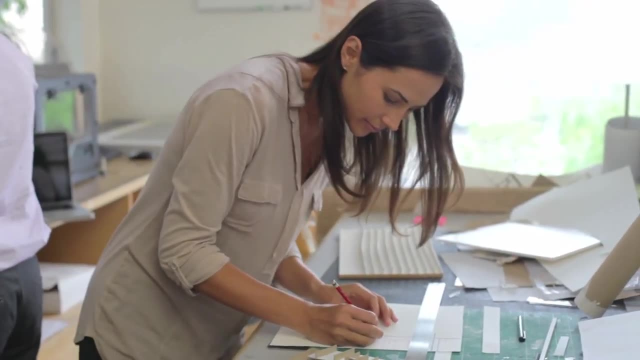 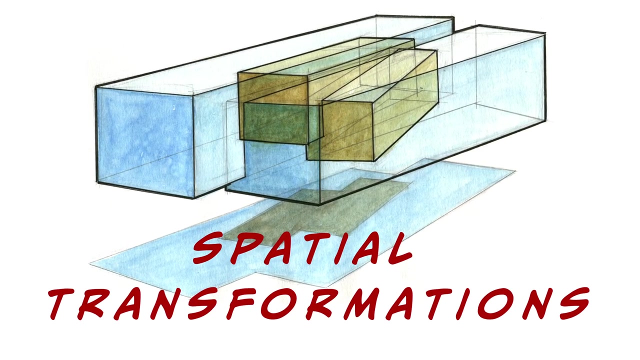 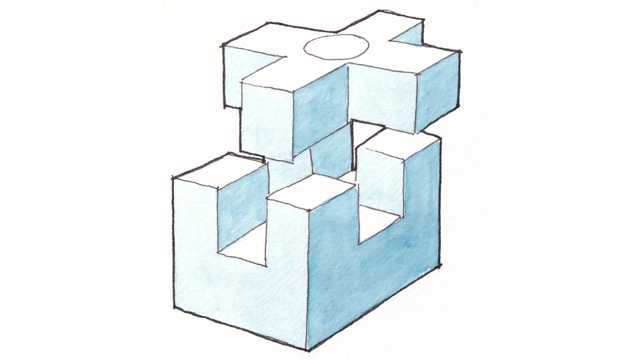 students can't understand basic spatial design. To address this problem, this video gives an overview of spatial design as it should be taught in architecture school. Let's get started. Spatial transformations: Spatial transformations can be understood as the transformation of primary solids through manipulation of planes of the volume. Geometric transformations: 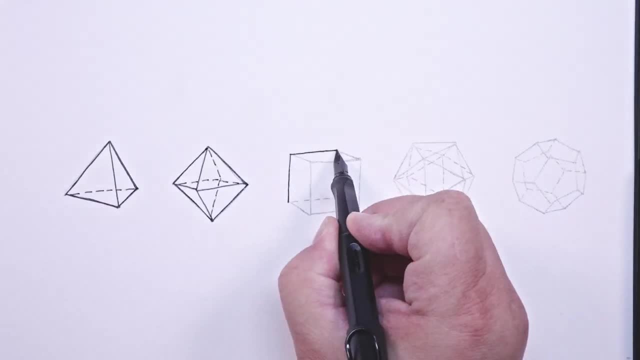 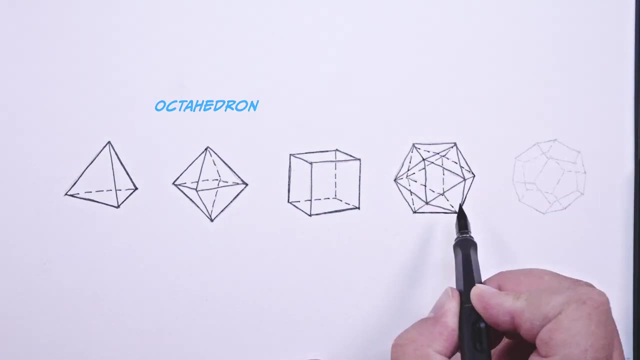 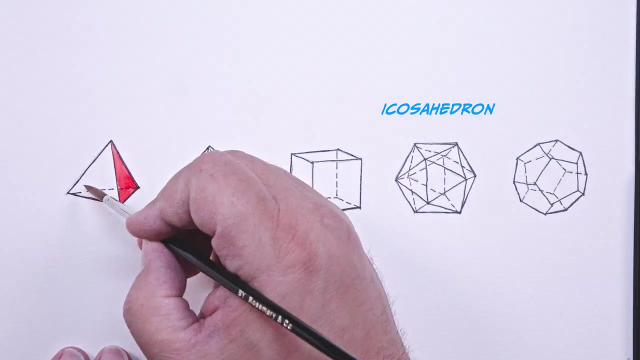 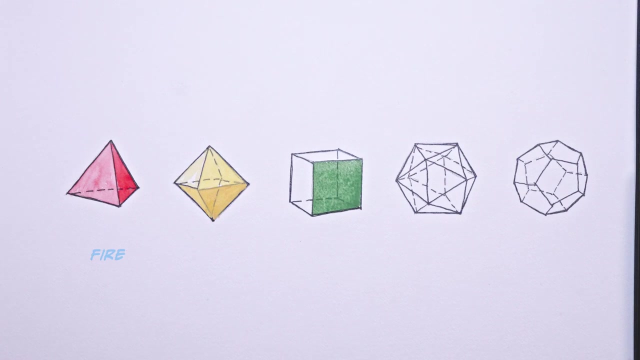 The mind naturally envisions primary solids like cubes, spheres and pyramids. These can be modified to give the appearance of transformation. In Roman and Renaissance architectural theory, geometry represented the building blocks of the cosmos, with the platonic solids being linked to music, numbers and forms of the universe. Geometric transformations. 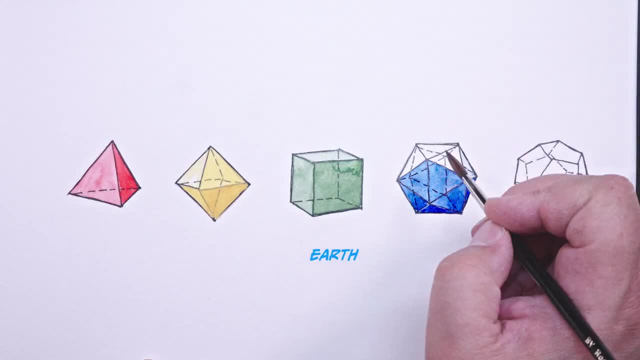 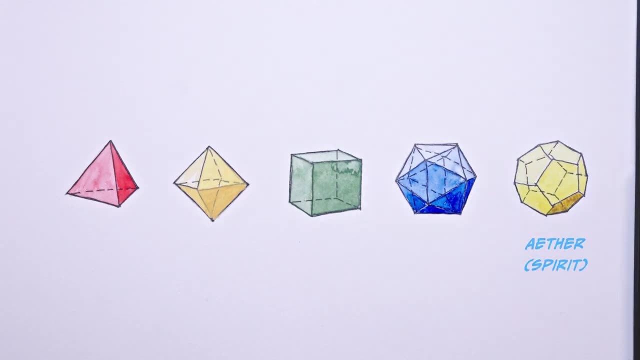 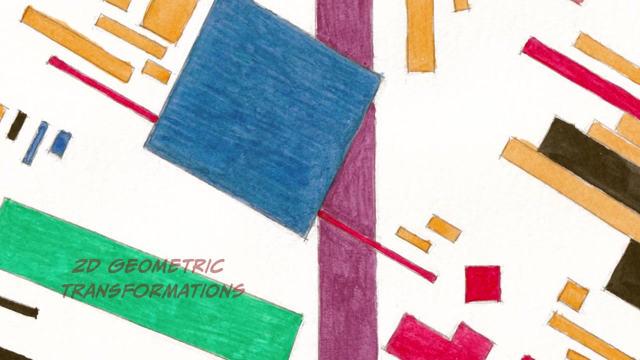 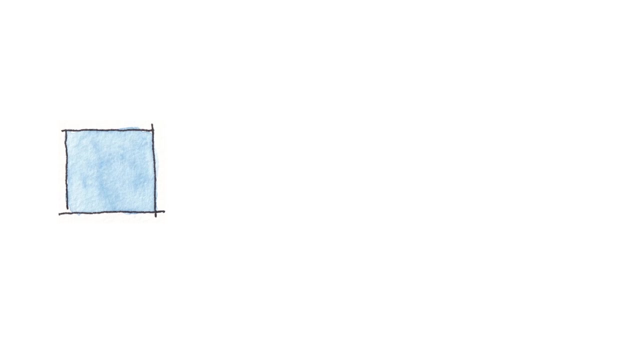 are accomplished using musical harmonic scales, number ratios and divine proportions. Sacred geometry and architecture represented the microcosm, while the universe of God represented the macrocosm. When thinking about manipulating the form of three-dimensional space, we can use all the methods of 2D geometry. The most basic is called translation. This means to move. 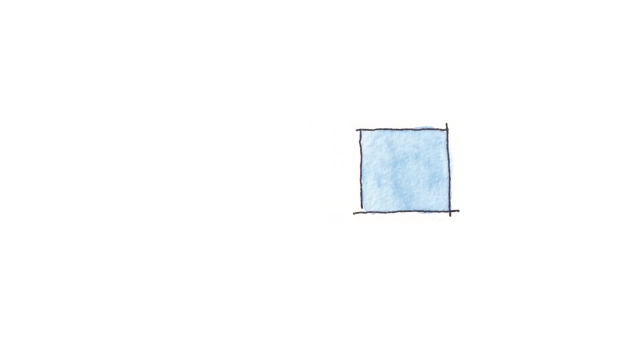 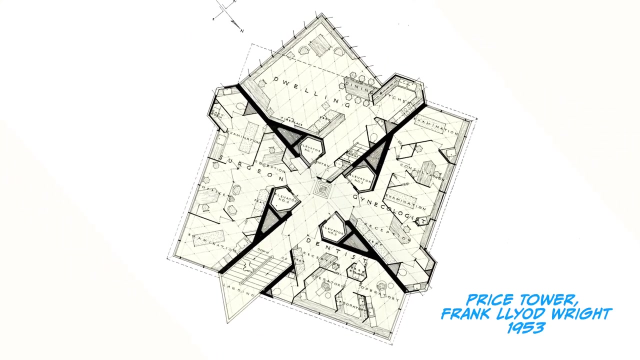 the position of the form. Although this seems basic, it is the most used transformation in design. Rotate: Another basic way to modify an existing geometry is to rotate it. This is the diagram for Price Tower by Frank Lloyd Wright. He rotates a triangle to develop the floor plan. 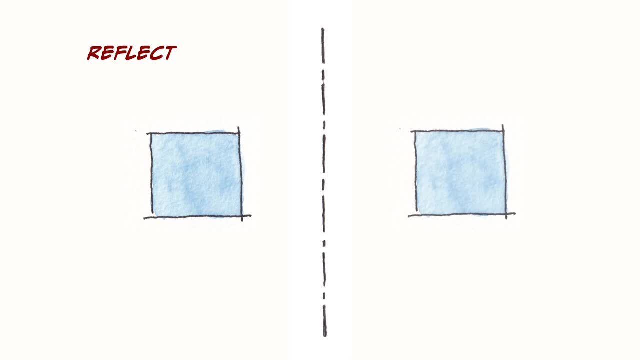 The third is to reflect the geometry. Here there is a center axis around which the form is reflected. The third is to rotate a triangle. Here there is a center axis around which the form is reflected. Here there is a center axis around which the form is reflected. An array is a. 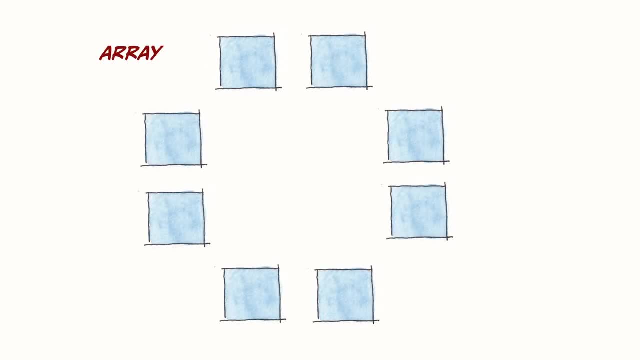 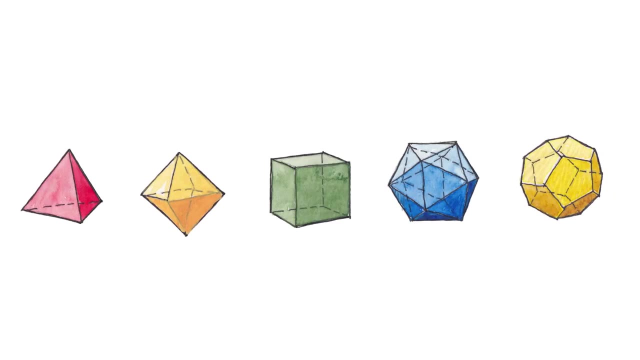 a repetition of a form in a certain way. Arrays can be linear, in a circle, in a grid, or three-dimensional. Dimensional transformation modifies a three-dimensional solid while keeping its identity from a family of forms. A cube can be dimensionally changed into a rectangular. 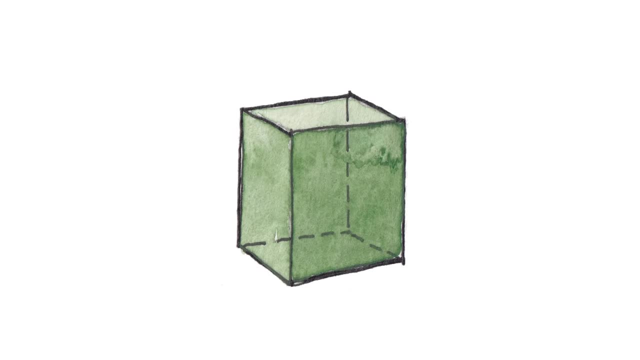 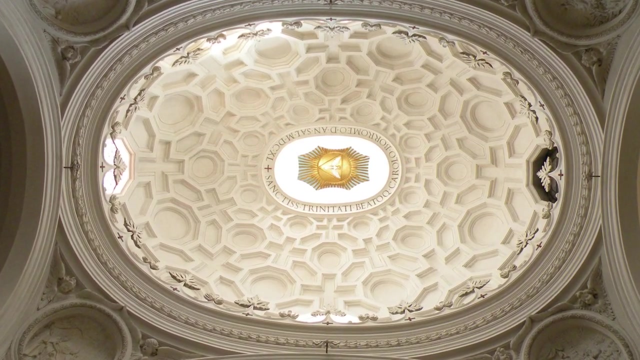 box, for example. A cube can be modified by transforming its height, width or depth. A pyramid can be transformed by altering any of its faces or sides. A sphere can be transformed by elongating it along its axis, turning it into an ellipsoid. 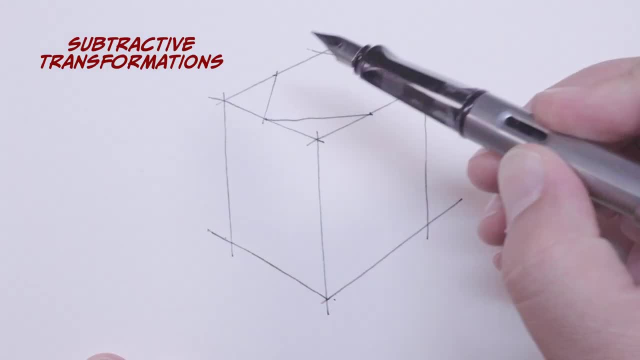 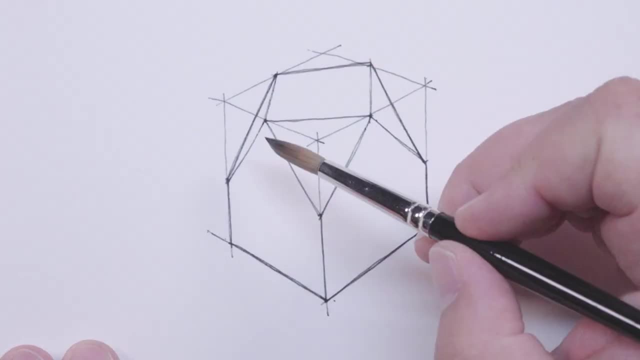 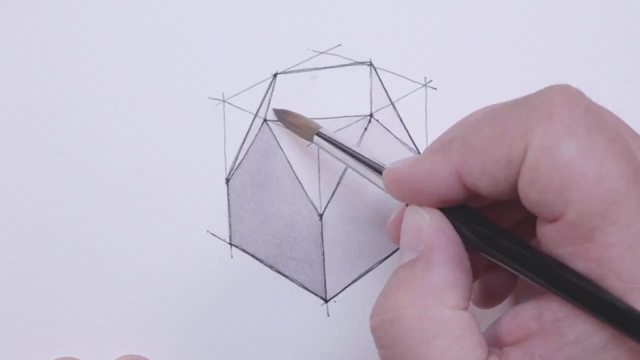 Subtractive Transformations. A form can be transformed by subtracting a portion of its volume. Words like carve or cut can be used to describe these transformations. Subtractive Transformations suggest the physical, physical act or gesture of cutting and removing. The human mind tries to always envision a 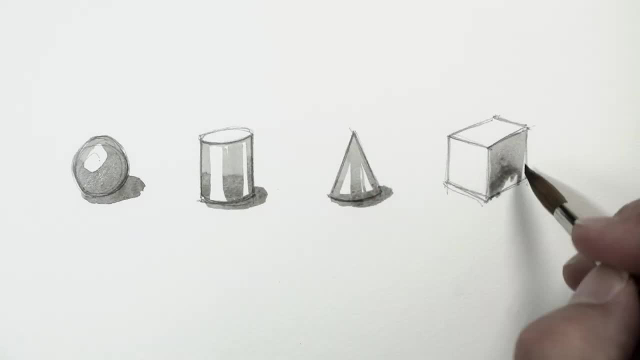 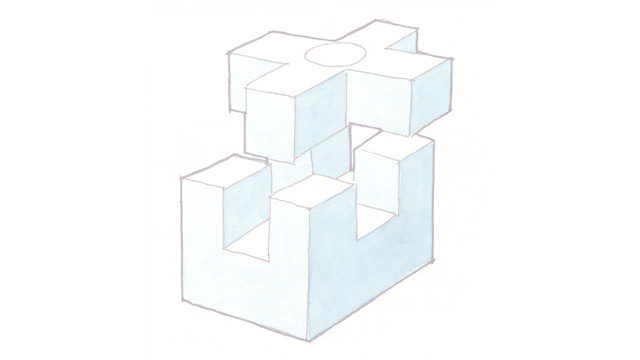 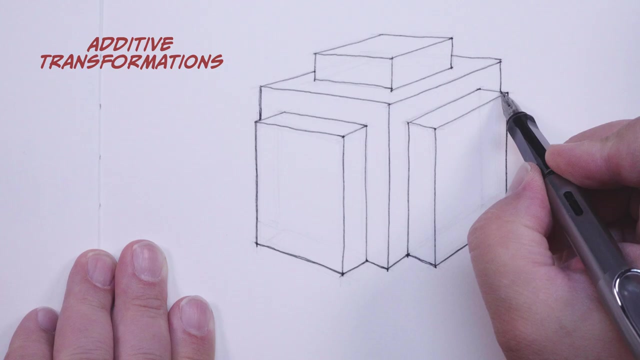 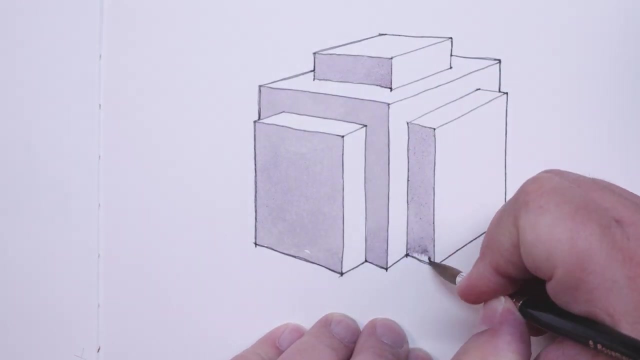 whole geometric object, like the primary solids. When the form is subtracted from, the mind still reads it as a primary form, but with a missing piece. Additive Transformations: A form can be transformed by the addition of elements to its volume. Additive form is produced by attaching one or more forms to 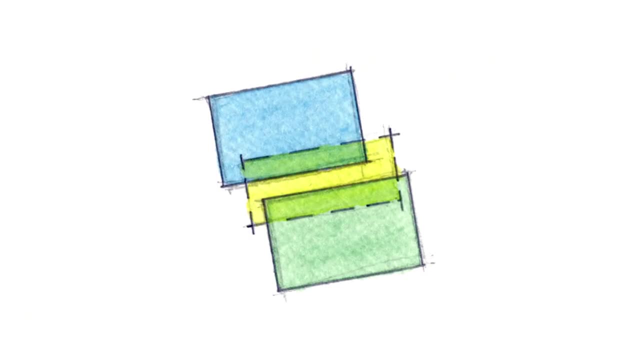 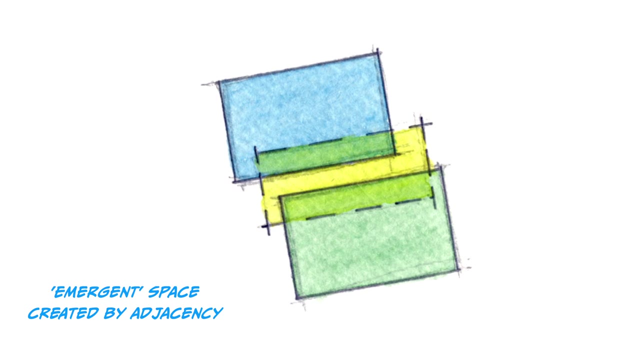 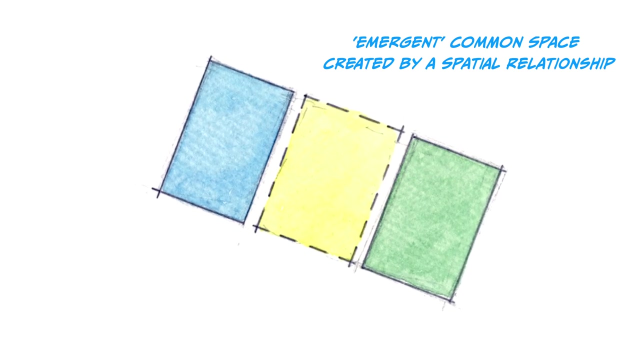 its volume. Additions may not touch. This is a relationship of two or more spaces that may relate to each other visually or conceptually, but do not physically touch. I call these spaces emergent space, as they emerge from the relationship between elements, Edge to Edge Contact. 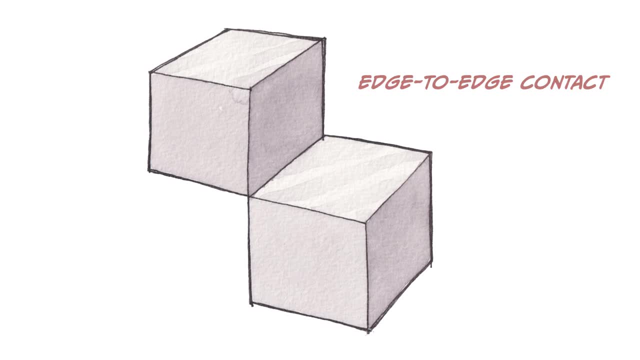 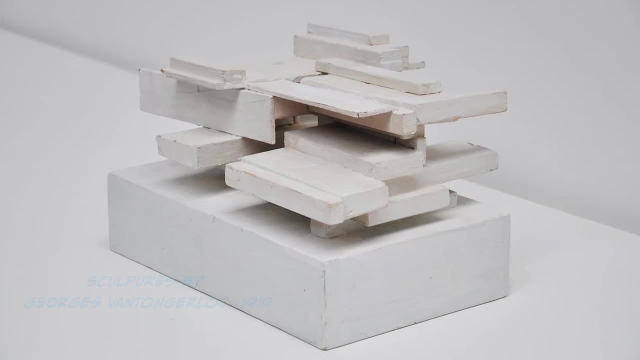 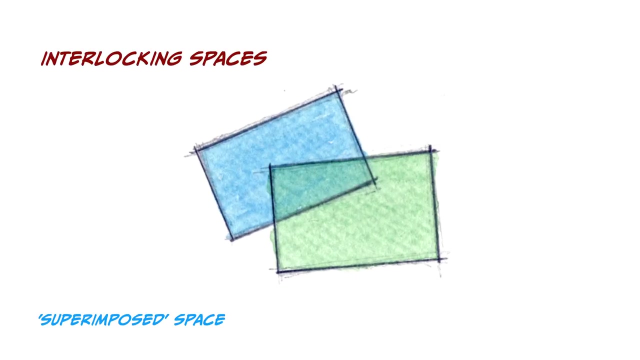 In this relationship. the forms share a common edge and can move or pivot around this edge. Face-to-face contact In this spatial relationship. forms share a common face and can move or transform around it. Interlocking volumes In this spatial relationship. 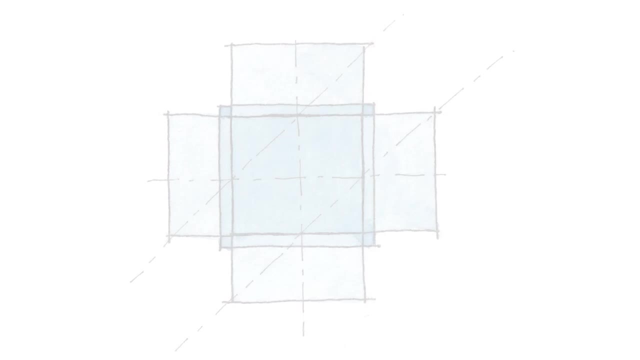 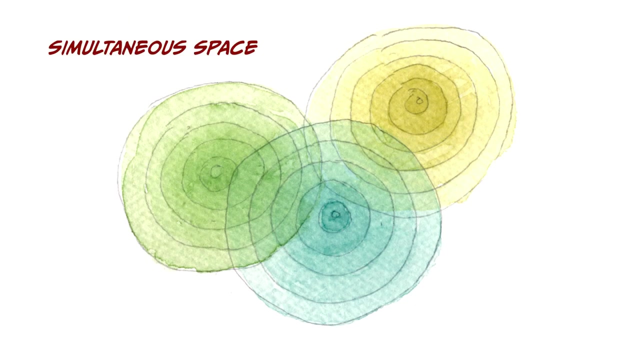 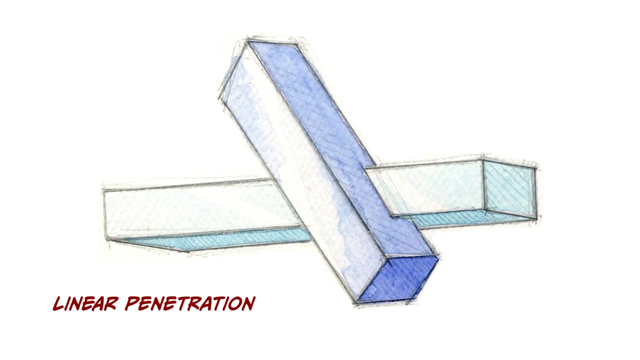 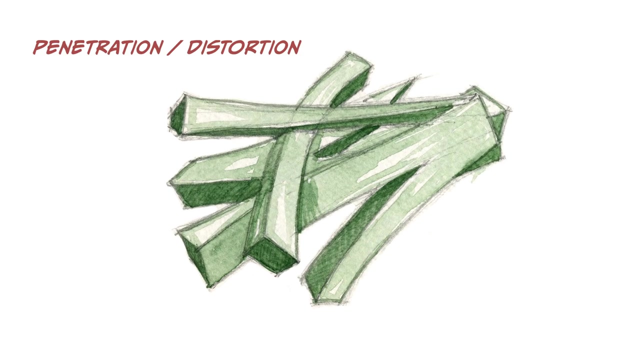 spaces interlock or overlap each other. This is by far the most used additive transformation, Simultaneous space. Architects' primary compositional tool is to create a relationship between spaces. Architects play with these relationships, sometimes overlapping spaces, sometimes designing adjacencies. 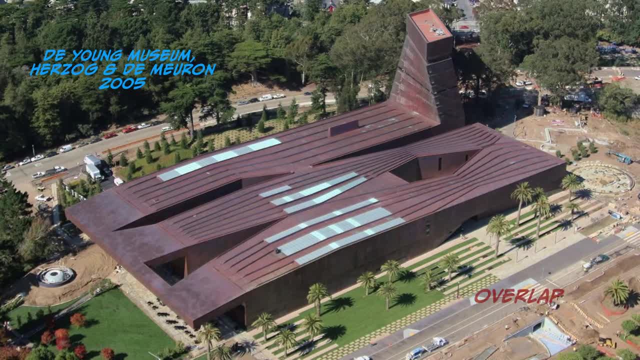 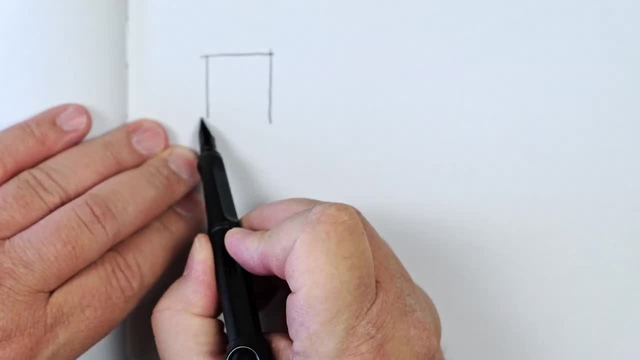 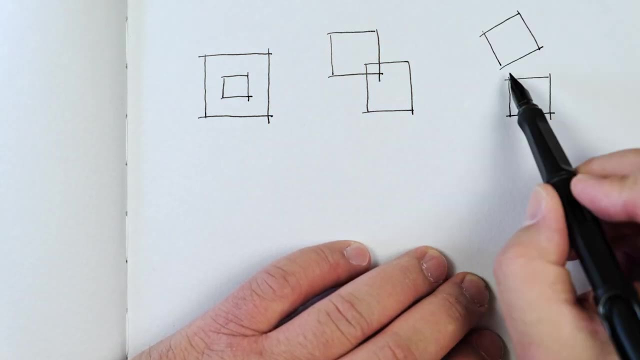 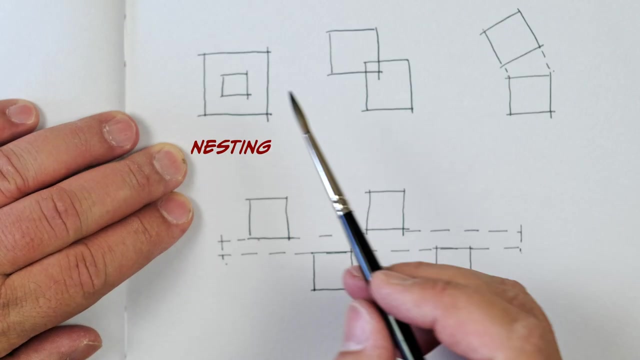 and sometimes linking or separating spaces. I call the act of creating relationships between spaces simultaneous space. Interlocking spatial relationships result when two spaces overlap, creating an emergence of a shared space. Each space retains its visual identity and definition as a space Nesting. 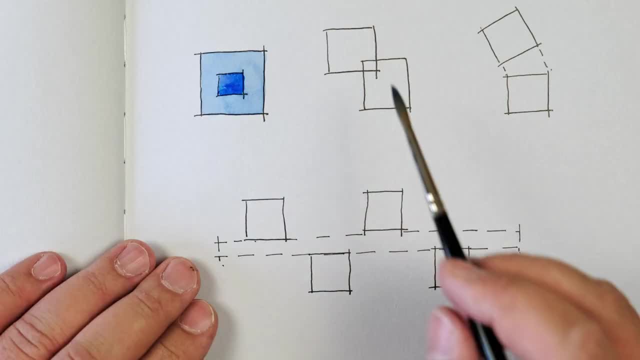 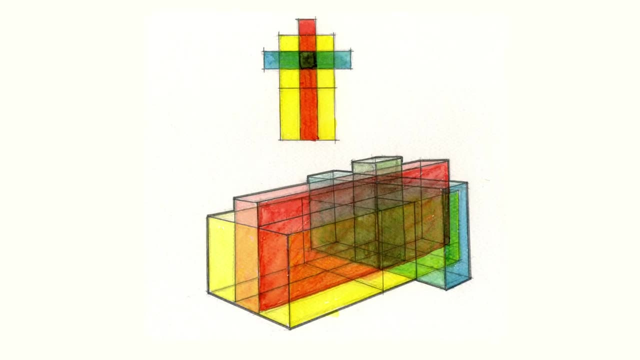 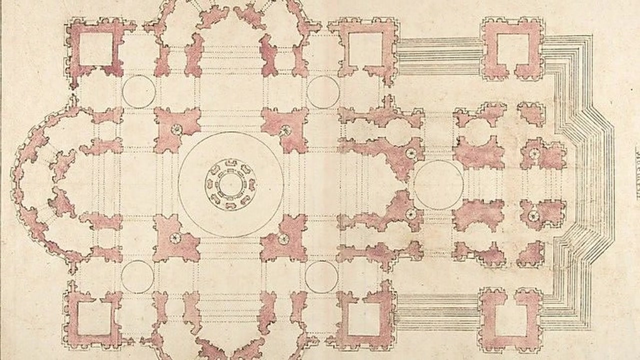 A space can envelop and contain smaller spaces within its volume. A visual and spatial relationship between the two spaces can be created. Nesting was most dramatically used in Roman and Renaissance architecture, especially in church design. In mid-century modernism, the open floor plan allowed for small spaces. 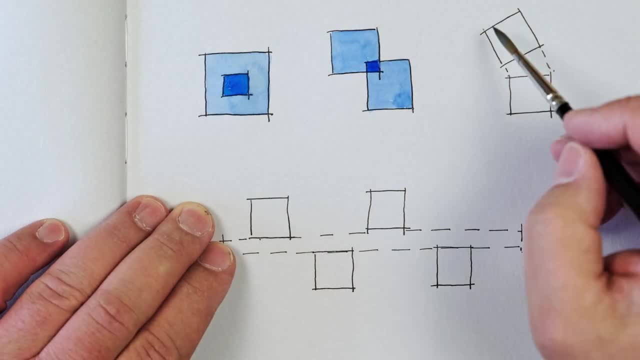 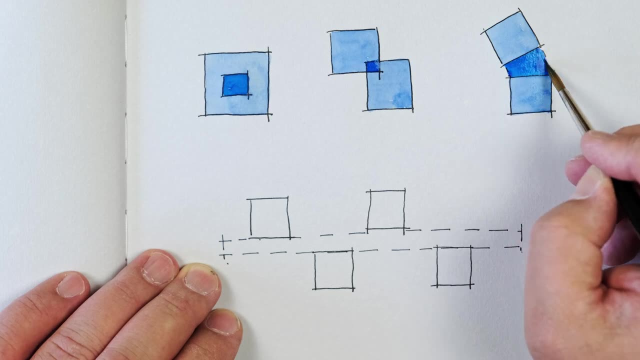 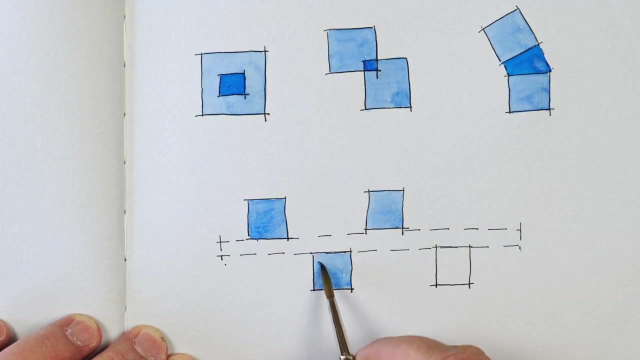 to nest inside larger ones. Adjacent spaces: Adjacency is the most common type of spatial relationship in architecture. Here two or more spaces are clearly defined and a new space emerges from the proximity to each other. Linked spaces: A form of adjacent space is the linked space. 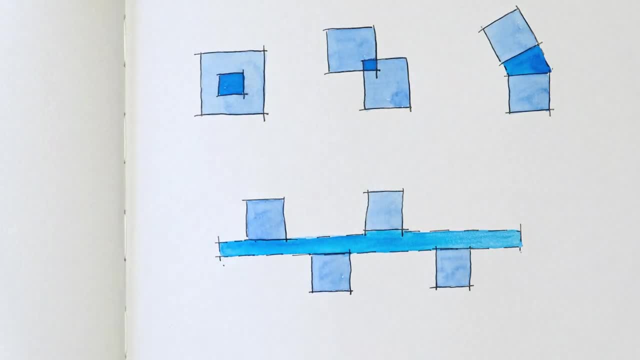 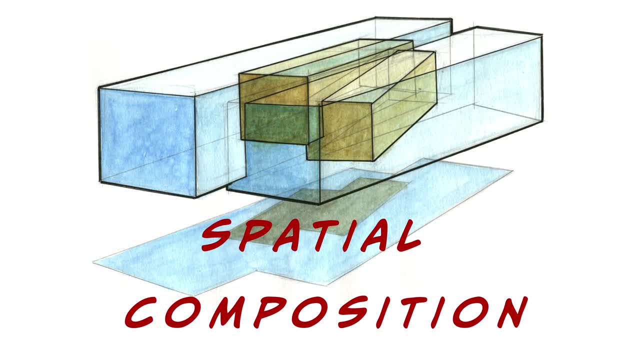 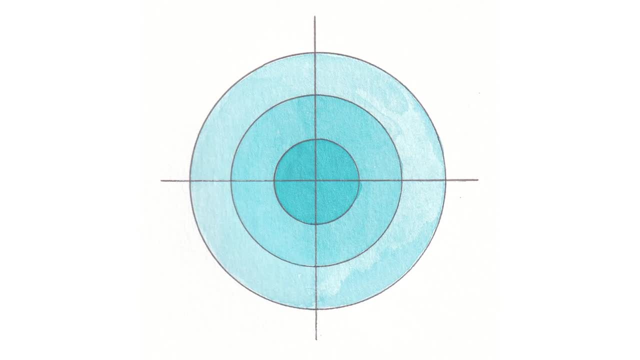 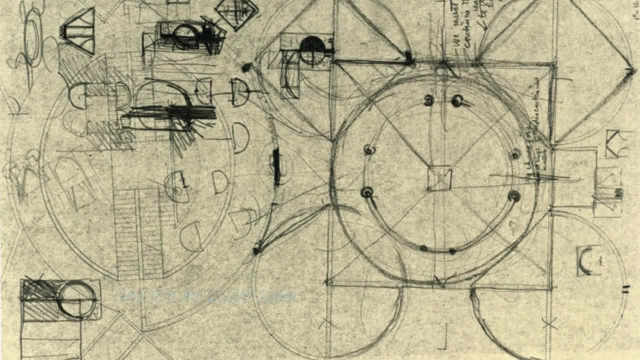 Spatial composition. Architectural space is always organized into a composition. A centralized space is the most basic spatial composition. Here space has a center and a periphery. Often there is a number of smaller spaces grouped around a larger, dominant central space. 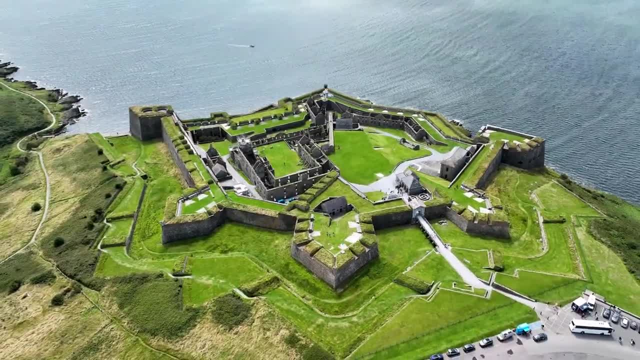 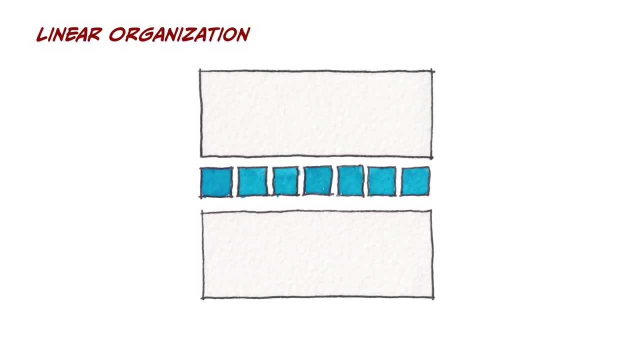 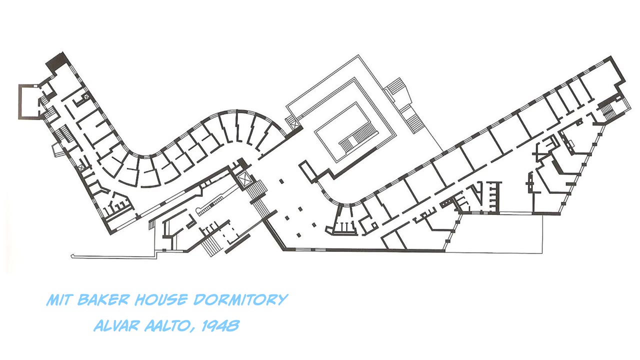 This is the most common form of city design, especially if the city grew naturally from its center. Linear space is another compositional tool. Here space is arranged sequentially in a row. A person moves through space after space in a path. Often these consist of repetitive spaces of the same size and form. 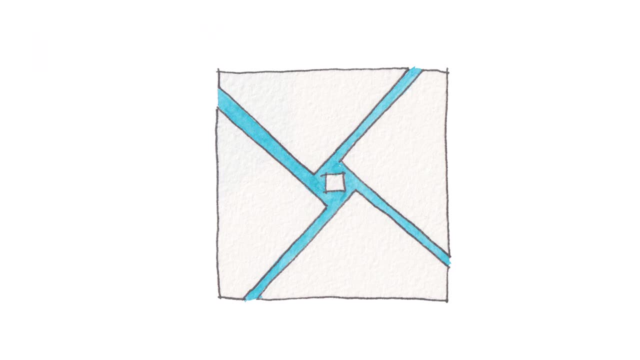 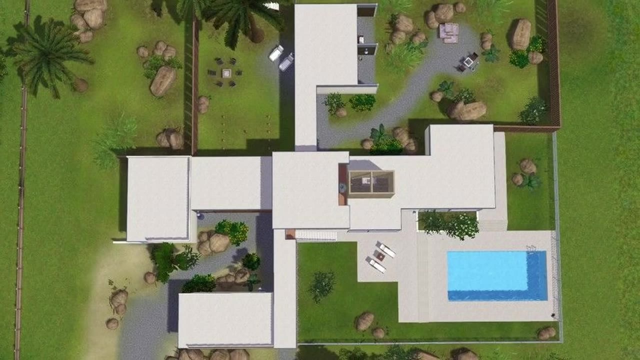 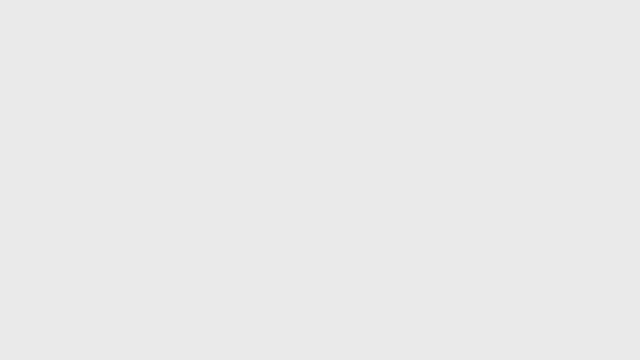 Radial space starts with a center and extends out to the periphery. It combines the elements of both linear and centralized organizations. This results in a dynamic composition that suggests a rotational movement around a central space. Clustered organization are spaces that are grouped together by proximity or a common identity. 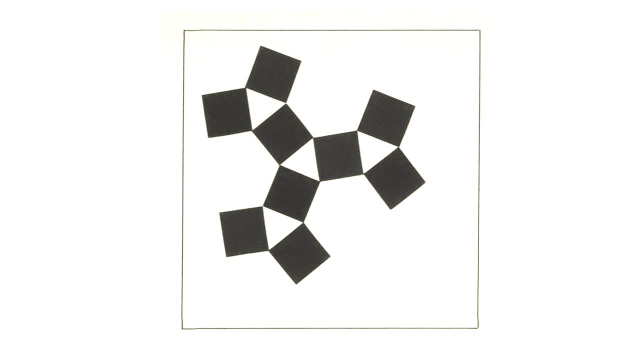 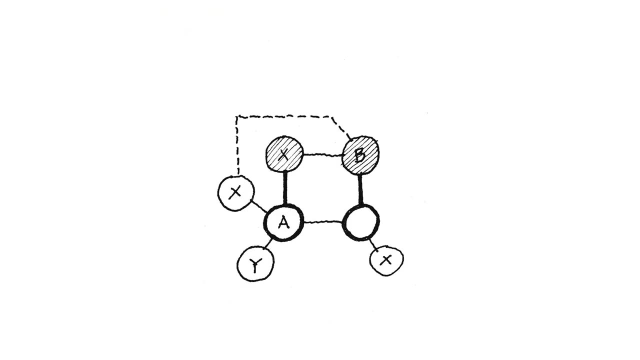 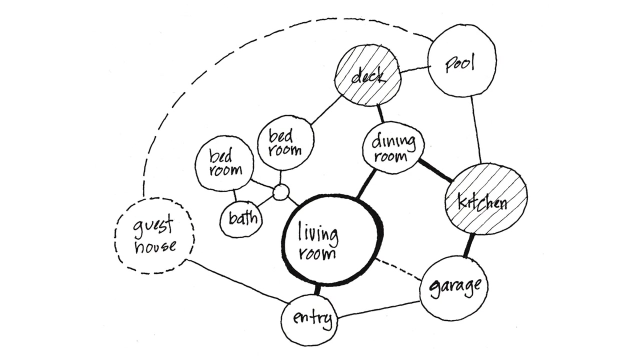 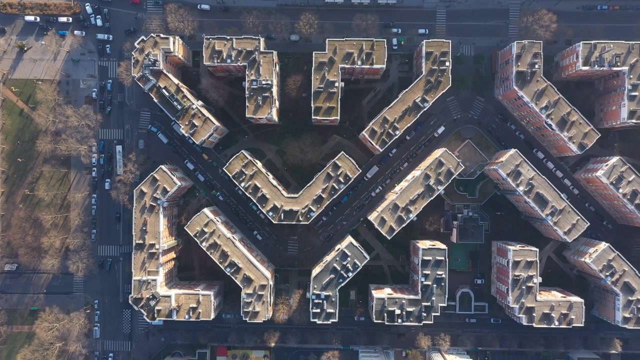 It often consists of repetitive spaces that have similar function or share common visual forms. In modernity, the term adjacency was used to describe a clustered organization pattern. Adjacency diagrams used functional proximity to compose spaces. Clustered organization can be combined with other ordering principles to create even more design possibilities. 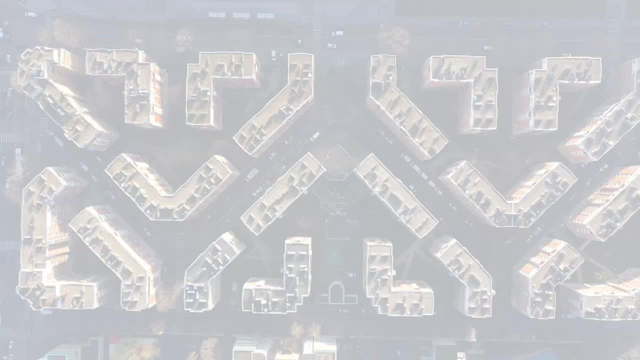 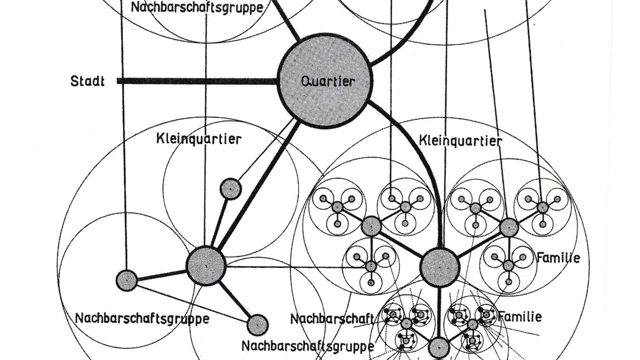 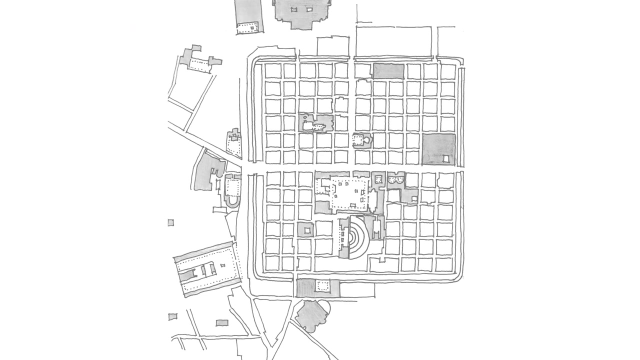 such as around an axis or along a path. They can be organized around a central form, they can be a space within a space and they can be symmetrical or asymmetrical. A three-dimensional grid can be used to organize space Forms. spaces and positions in space can be regulated by a two- or three-dimensional grid. 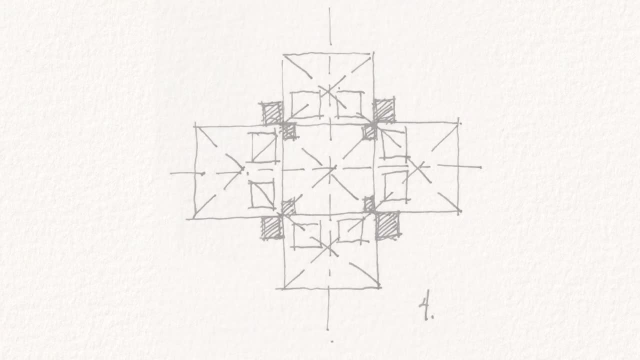 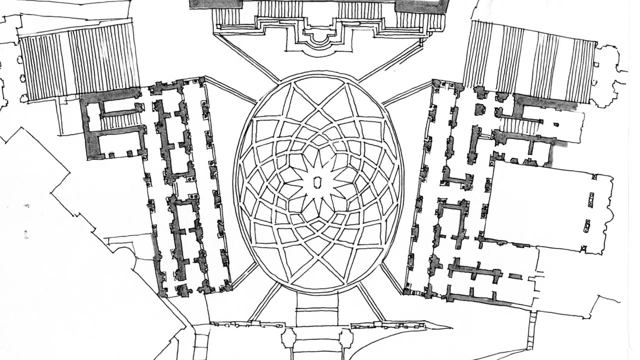 Grids can be used to organize spaces, but they can also be used to modify and transform space. Grids don't have to be regular or even square. They can be triangular, octagonal or even circular. Peter Eisman often played around with. 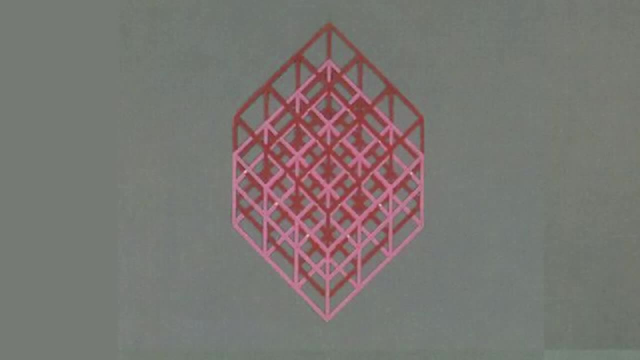 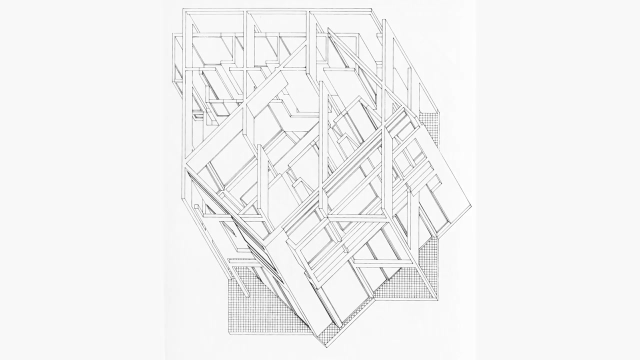 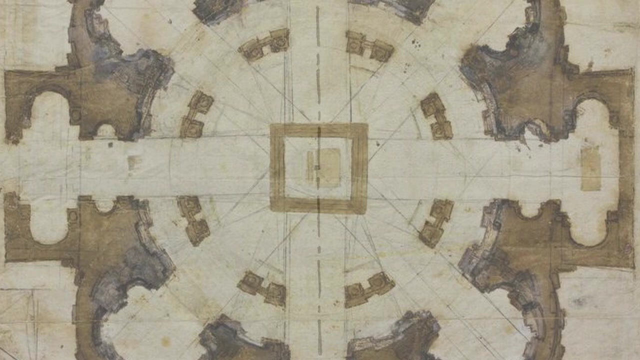 three-dimensional grids, juxtaposing them with spatial or structural elements of the building. For Eisman, the grid, instead of organizing space, disrupts it. An axis is a central line that bisects a space into two symmetrical spaces. Symmetry reflects a group of spaces around a center axis. 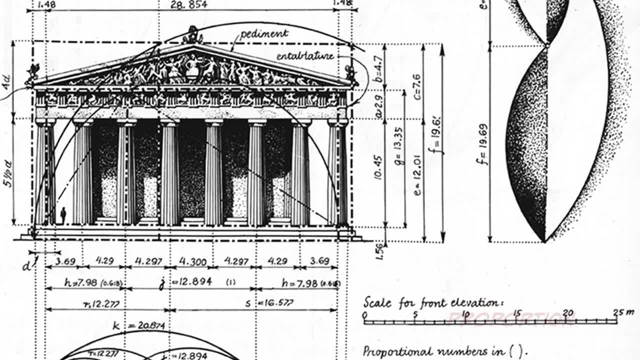 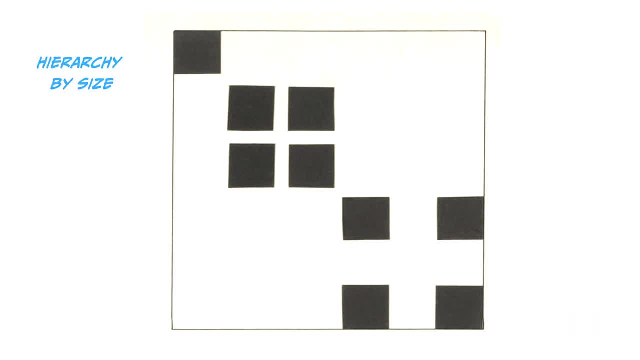 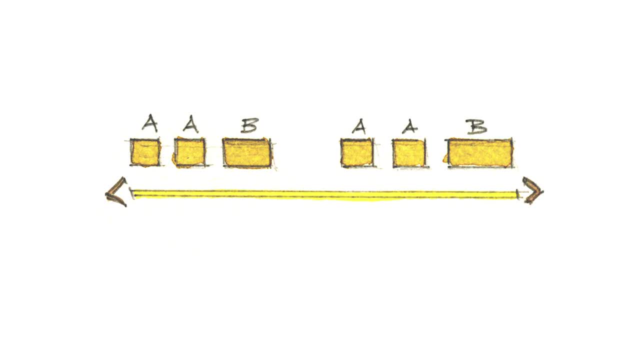 Proportion is a relationship of the parts to the whole or the parts to other parts. Hierarchy is a system of spaces ranked by order of importance. Rhythm is a pattern of spaces with repetition or alternating patterns of elements. Repetition is the act of repeating a space in the design. 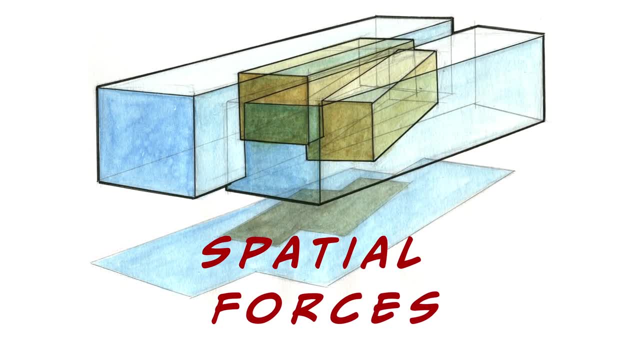 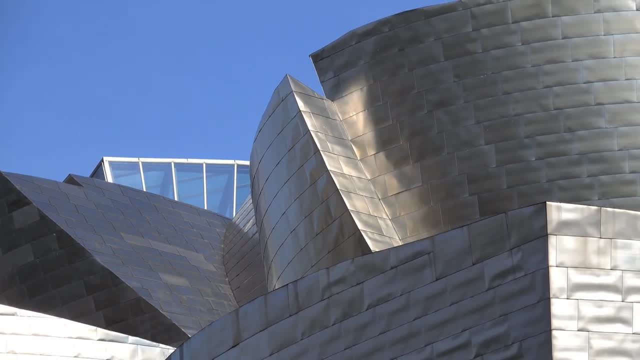 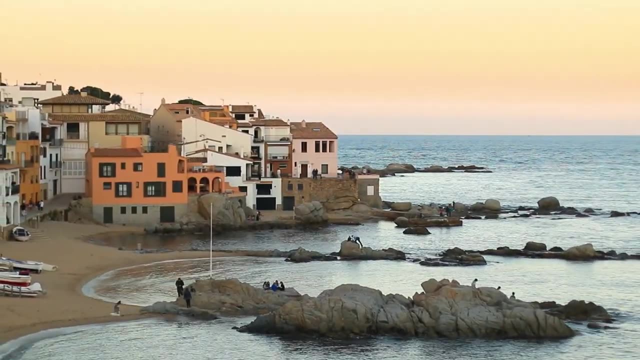 Spatial forces. Formalism, abstract form-making shouldn't control the final shape of a building. Rather, the form should arise naturally from the forces that shape it. Form arises as a response to contextual forces. It should not arise from pure form-making. 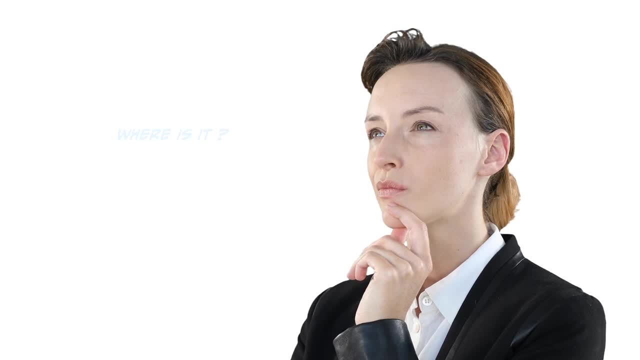 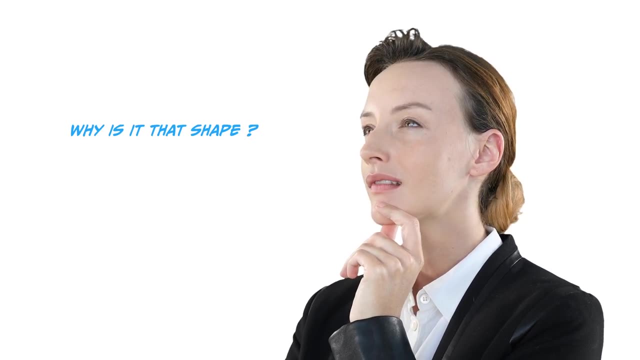 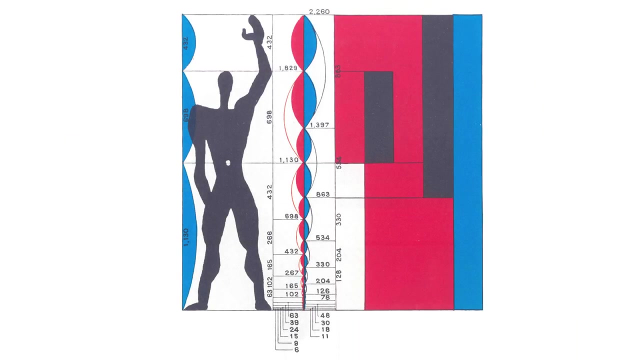 To discover the context, an architect must ask: Where is it? What size is it? In other words, what is its scale? Why is it that shape? How is it that shape? In other words, how is space structured? Architectural modes of representation that don't address scale. 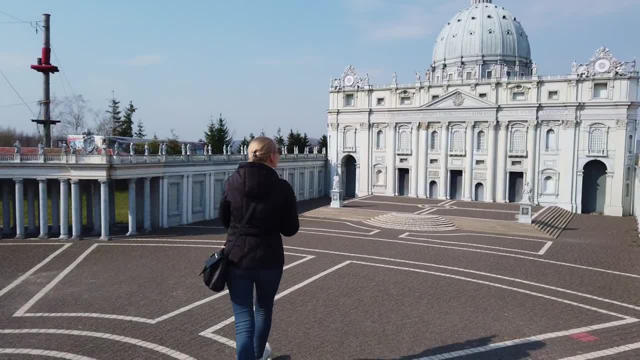 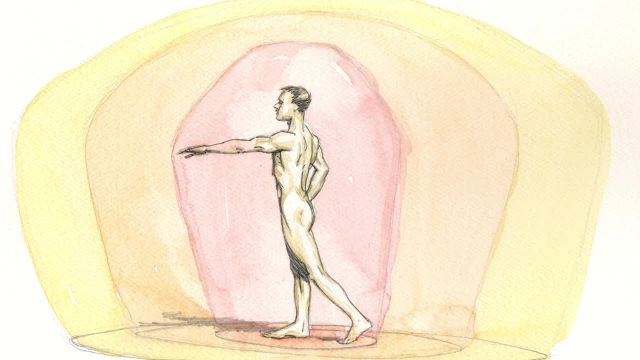 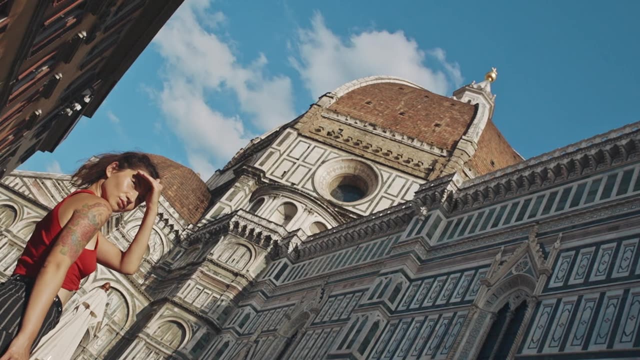 are, at best, incomplete and, at worst, bad architecture. How the human body is deployed in space should be a primary concern of architectural design. Space is a lived experience and the design of space needs to address this experience. Unlike computer models, real-world architecture is shaped by gravity. 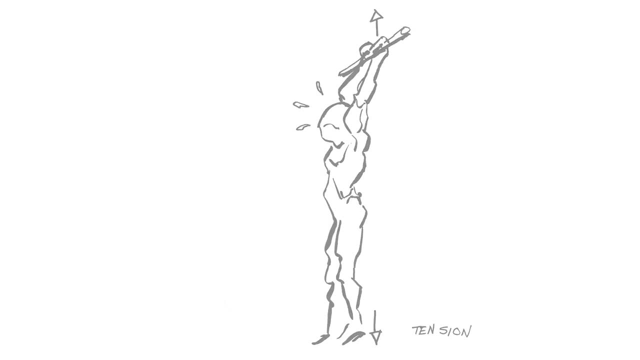 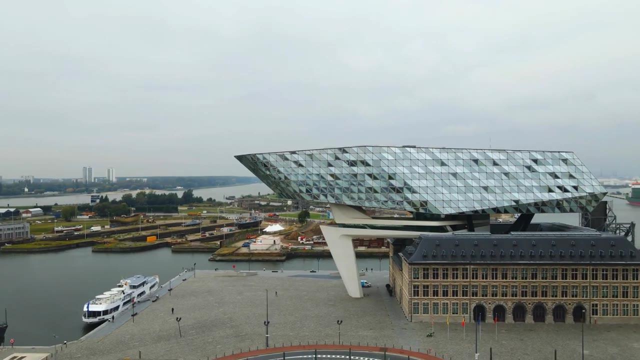 There is always an up and a down to space. A space can conform to this force and be a simple one-step structure, or it can defy gravity and appear to float in the air. Either way, a space must have a response to gravity. 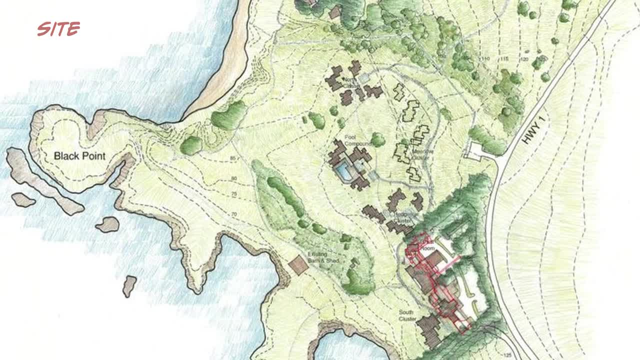 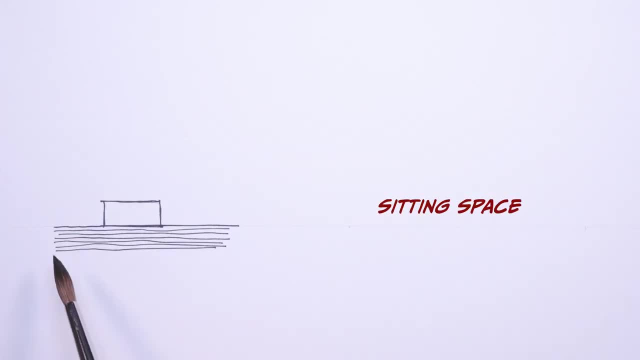 One of the most important relationships a building form can have is with the ground plane. Sitting on the ground is the simplest relationship with the ground plane. Here the building sits on a slab on grade. The next relationship a space can have to the ground is to dig into it, causing a. 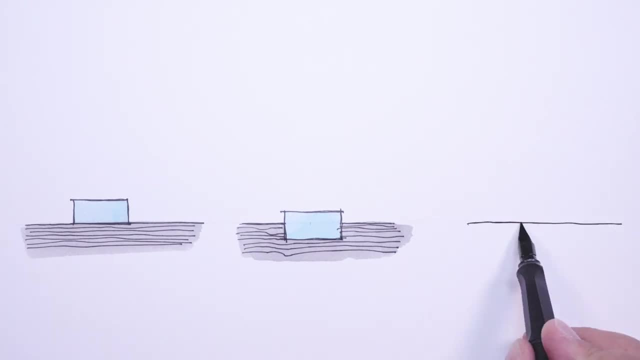 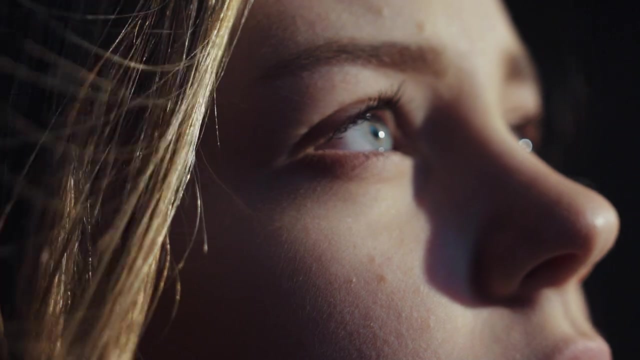 depression. Space can also hover above the ground plane as though gravity had no effect on it. Space appears to float weightless above the ground. Light defines and creates space From the exterior massings of space to the interior space. light is used to shape and reveal space. 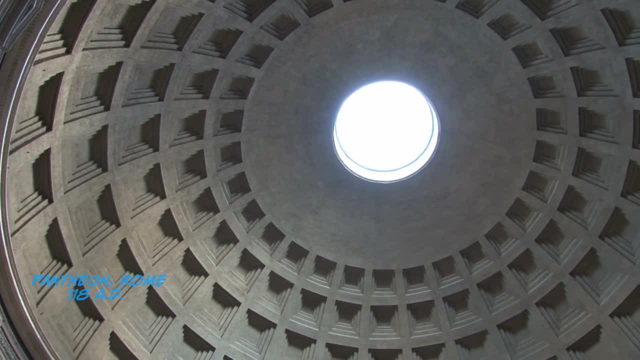 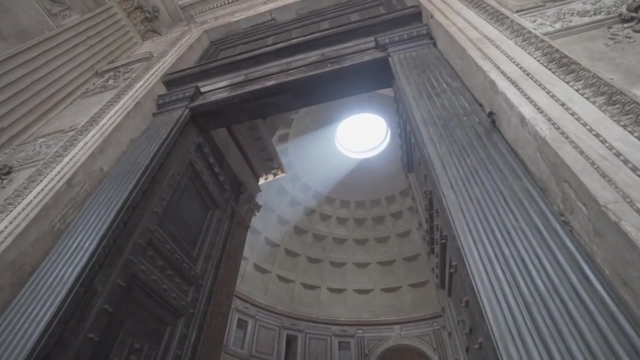 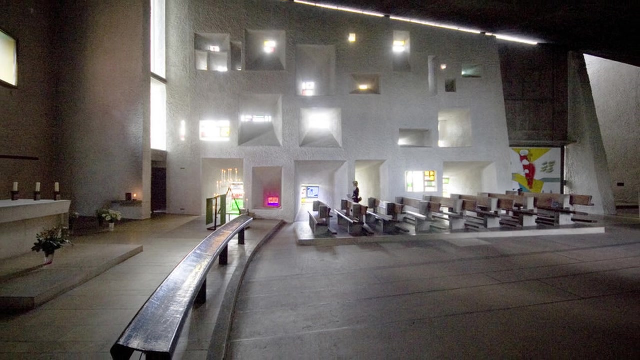 As such, architects use natural light from the sun to shape space. This is ever-changing, based on the movement of the sun through the sky, rising in the east, setting in the west and in the northern hemisphere, traveling around the building from the south. Space must always interact with the forces of sunlight across the sky. 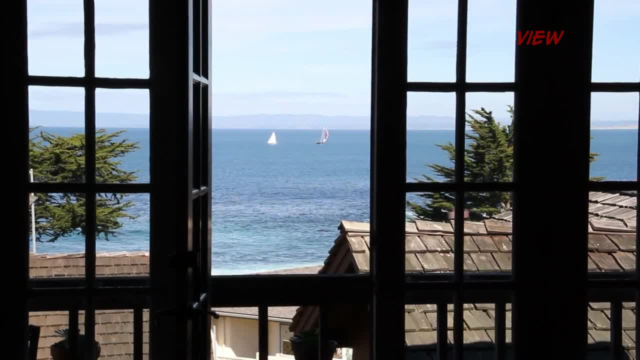 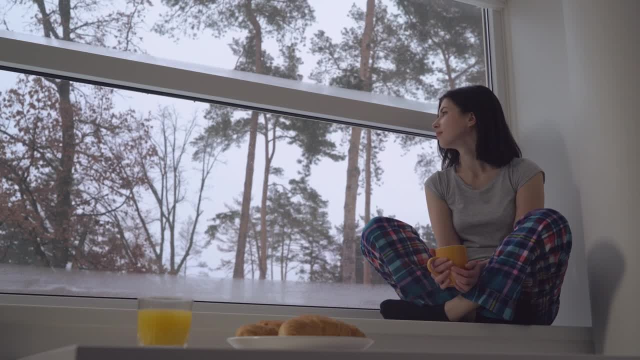 Interior space is transformed based on a person's view to the outside. Often, this is thought of in terms of windows and framing the view, But what an architect is actually doing is setting up the relationship or experience between the inside space and the outside space for the inhabitants. 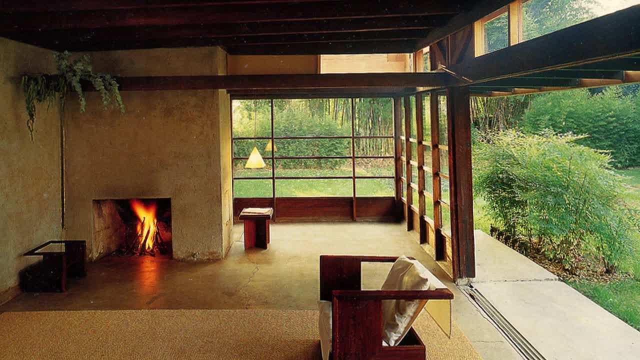 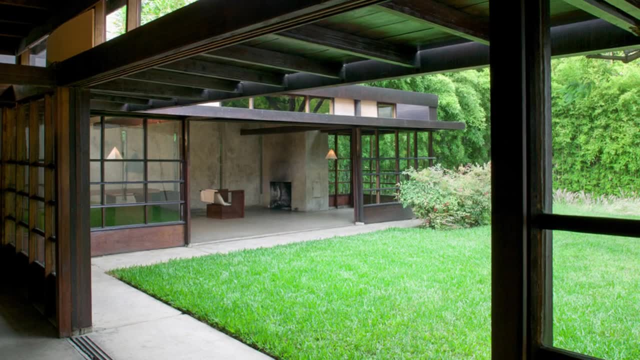 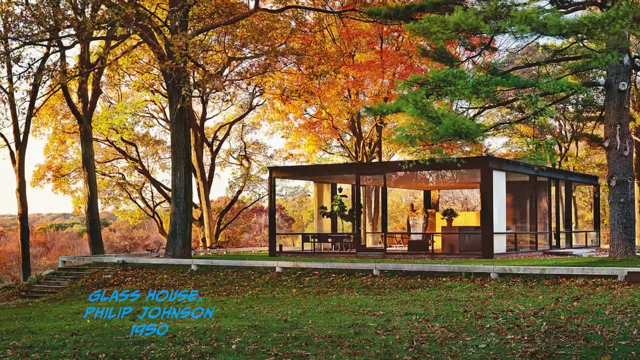 Views can be controlled or open, often based on the window or enclosure size. Many of the mid-century modern spaces explore the continuation between inside and outside space through the creation of an open view. Philip Johnson's glass house is perhaps the most famous example. 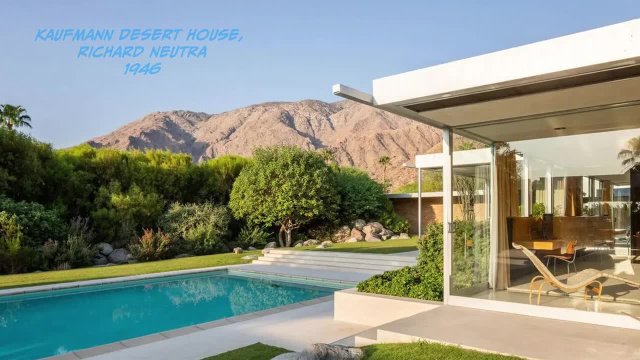 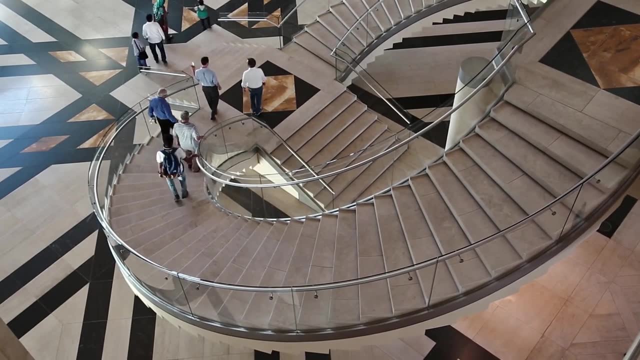 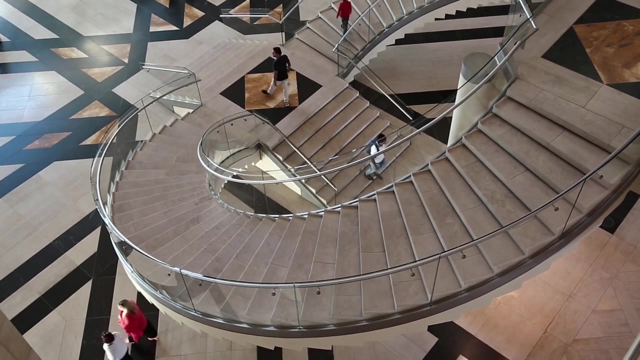 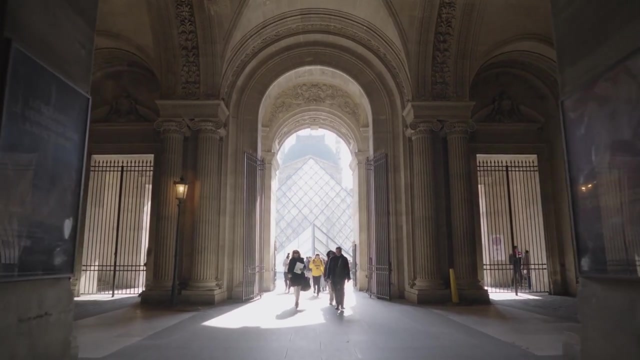 but Richard Neutra and Rudolf Schindler's works define California modern architecture. Circulation is also a force defining space. The architect can set up patterns of circulation through spaces. Also important in circulation is remembering where you were and thinking of where you are going. A person must be able to visualize spaces and remember them well enough. 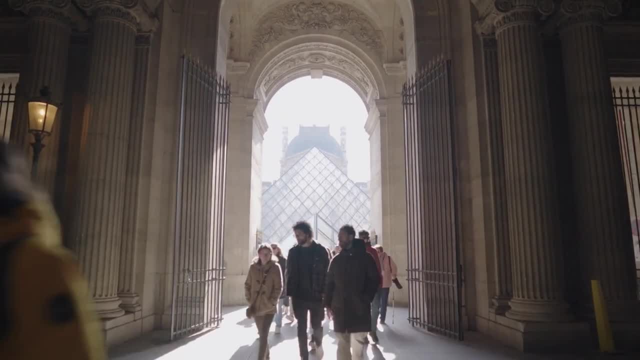 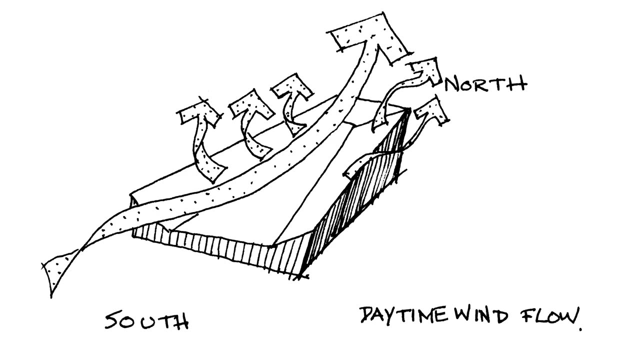 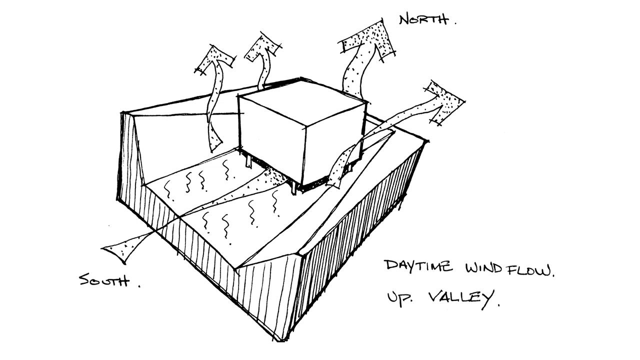 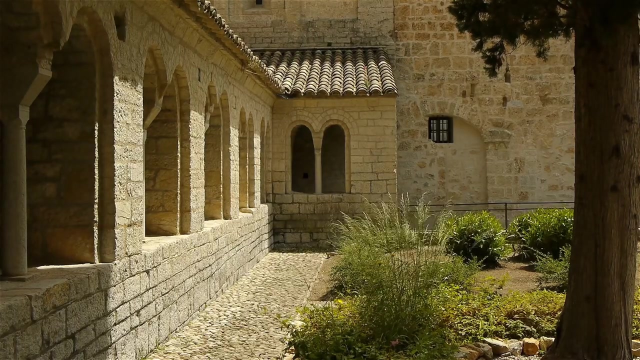 to move through them without getting lost. Wind is a force that is often forgotten in modern architecture. Before buildings had HVAC systems and were totally closed off from the outside, wind played a significant function in designing space, especially in hot climates. Courtyards used in the Roman house or in Spanish architecture were used to pull in cold air. 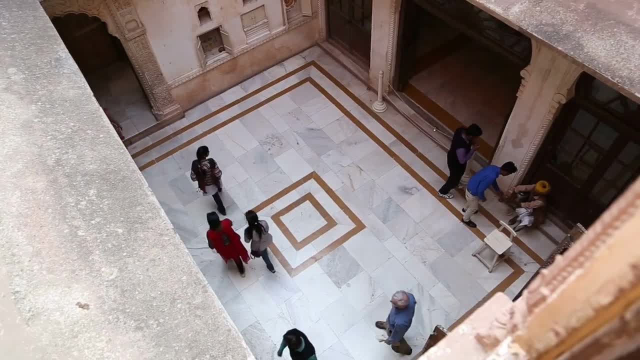 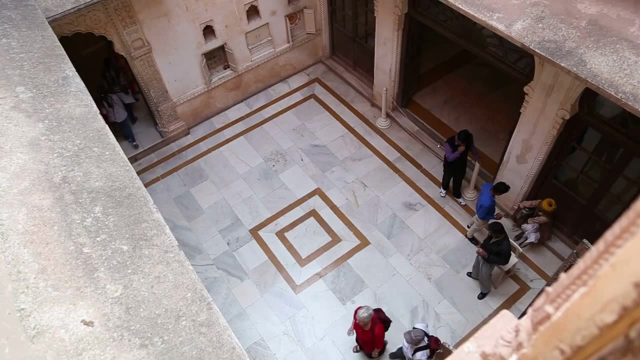 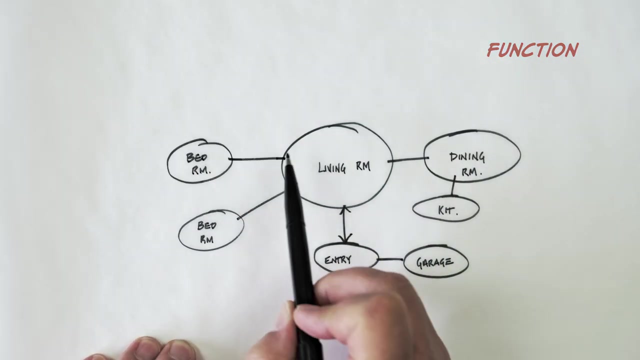 and keep the house cool in summer. Many traditional building types were designed around wind, either blocking it in cold climates or pulling it in in hot climates. Function can also shape a building. Modern architecture is based on form follows. function is often used to shape space. 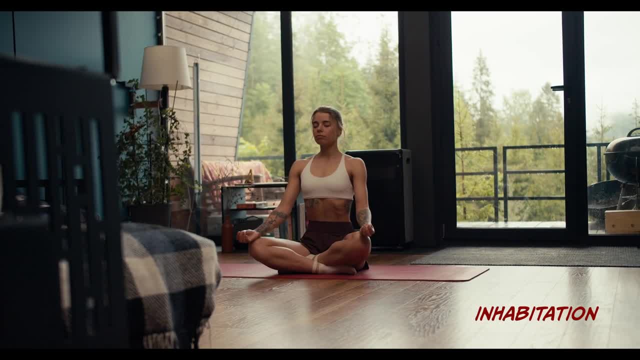 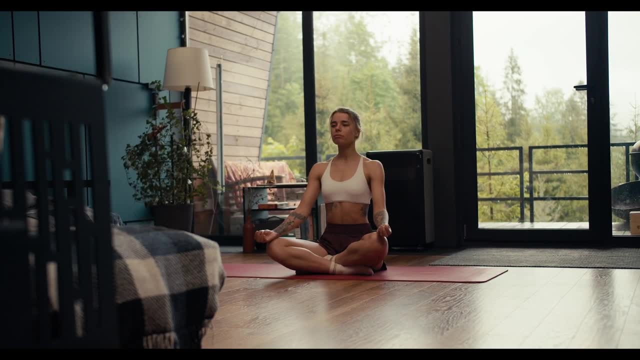 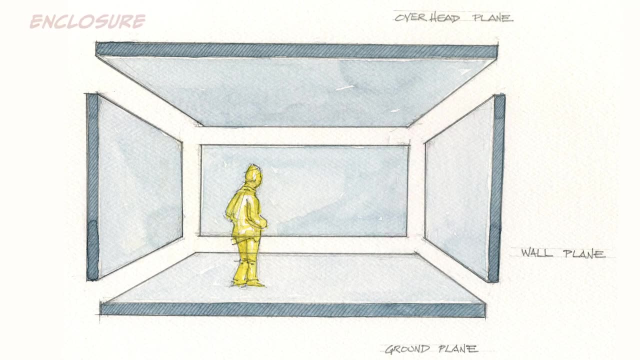 How people inhabit a space is a primary shaper of space. We often call this functional design, but on a more elemental level it is about life and how people actually use a space. How space is enclosed helps shape space. Architects use ground planes, ceiling planes and wall planes to shape space. 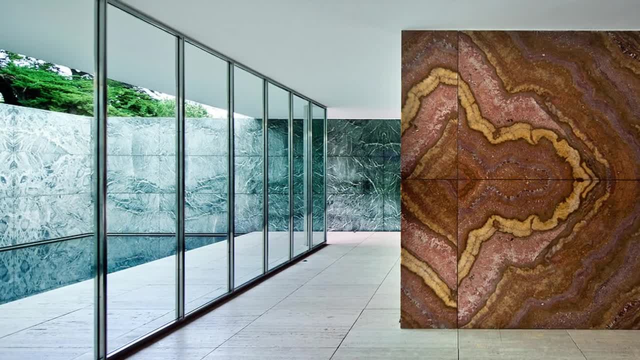 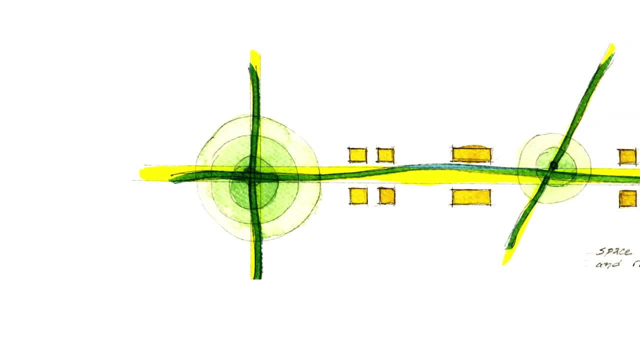 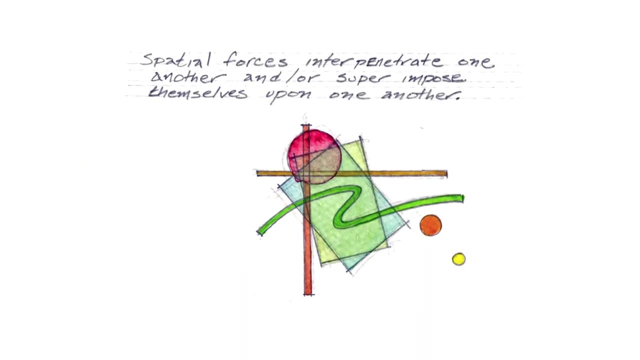 In modernism, the wall planes were played with and removed to create flowing spaces. In this video, I have tried to show how space is a verb, not a noun. Architects transform space and communicate this to the inhabitants. Space is not static. It should be used to communicate.